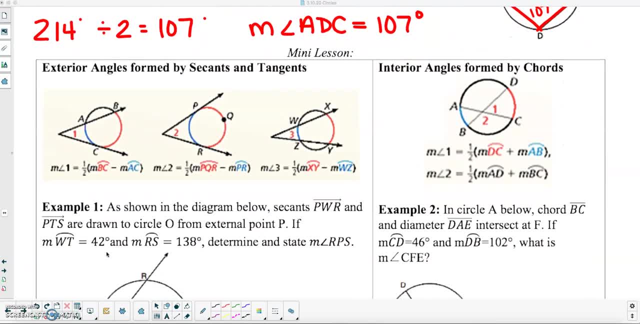 middle of the diagram, we're going to be talking about the angle ADC. So if you look at our beginning lesson, we're going to be talking about exterior angles formed by secants and tangents, as well as interior angles formed by chords. They are very similar concepts. 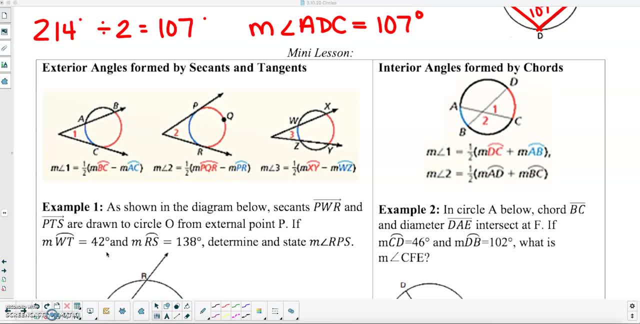 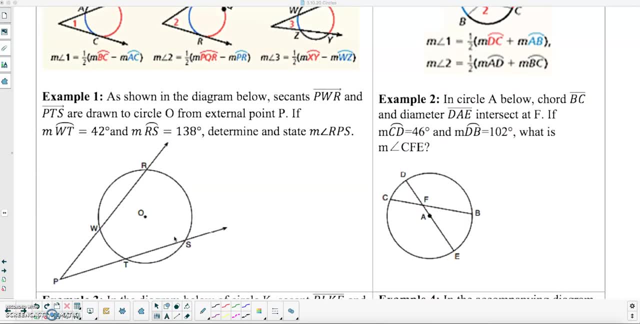 here. For the exterior angle, you're going to actually subtract the arcs, whereas for the interior angles we're going to add them together. So let's look at example number one. As shown in the diagram below, secants PWR and PTS are drawn to circle O from external. 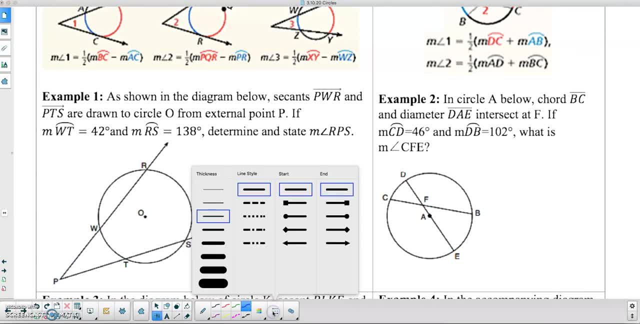 point P If arc WT is 42 degrees. so as I'm reading it, I'm going to write this into my diagram- and the measure of arc RS is 138 degrees. we are looking for the external angle of RPS. So because it's an external angle here, we are going to take the big arc, subtract the. 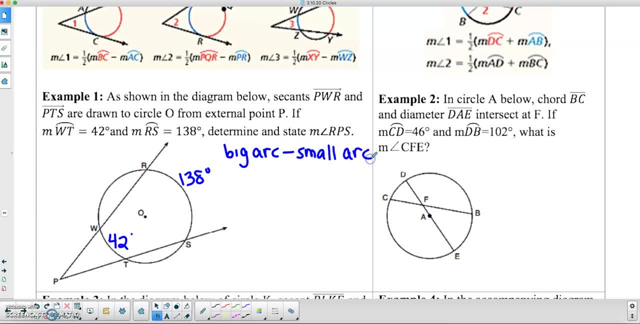 small arc and then divide it by two In order to get our exterior angle. So in this case, angle RPS is going to equal the big arc, which is RS, minus the small arc, which is WT, and then divide that by two. 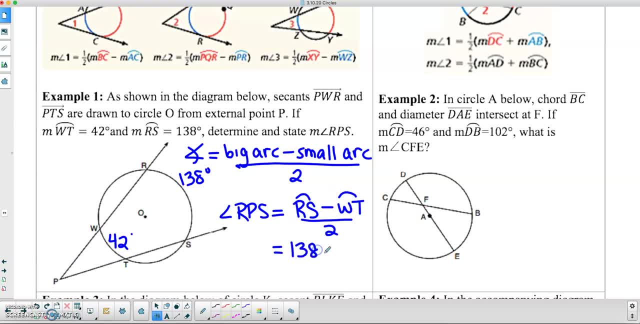 So we're going to substitute in 138 minus 42, and divide that all by two. Well, 138 minus 42 is RPS, So we're going to subtract that by two And then we're going to divide that all by two. 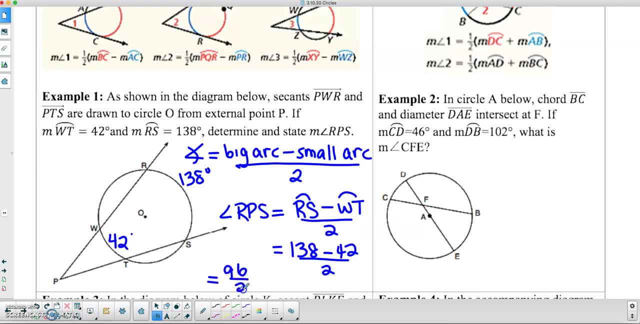 96, and then 96 divided by 2 is 48 degrees. So in this case, the measure of angle RPS is 48 degrees. Now looking at the next example, these are your two chords. So instead of subtracting, 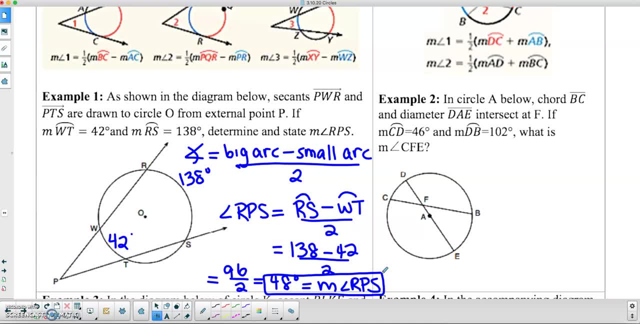 the arcs. we're actually going to add them together. So example 2.. In circle A below chord BC and diameter DAE intersect at F If the measure of arc CD is 46 degrees- so I'm going to label this here as 46 degrees- and the measure of arc DB is 102,. what is?